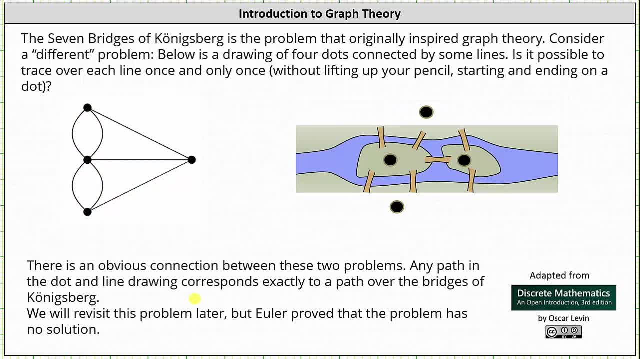 There's an obvious connection between this problem and the Seven Bridges of Konigsberg problem. Any path in the dot and line drawing corresponds exactly to a path over the Bridges of Konigsberg. Looking at the image of the Bridges of Konigsberg, 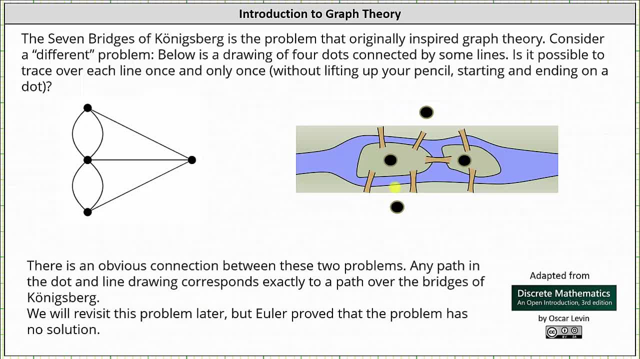 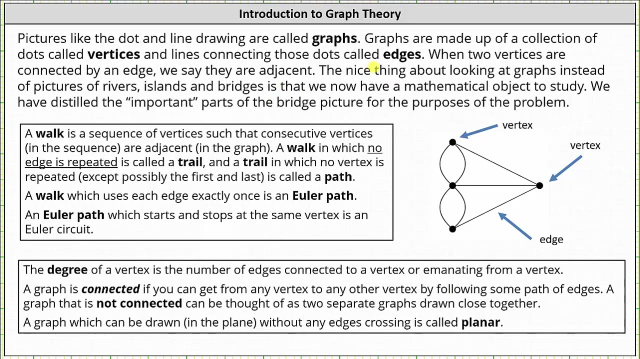 notice how I placed four dots on the four landmasses. From here, if I draw lines connecting the dots passing over the bridges, the two graphs are equivalent. And now let's talk about some definitions. Pictures like the dot and line drawings are called graphs. 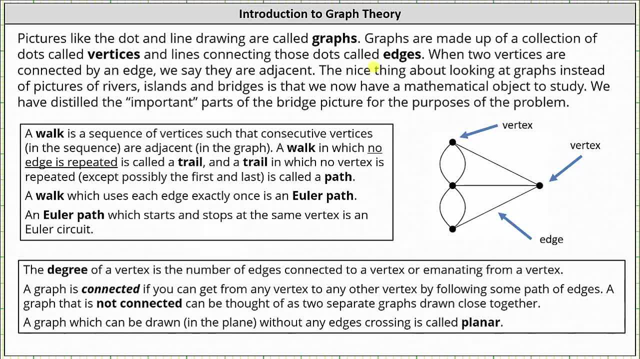 Graphs are made up of a collection of dots called vertices and lines connecting those dots called edges. Looking at the graph here on the right again we have a set of vertices and a set of edges. Vertex is singular for vertices. When two vertices are connected, we say they are adjacent. 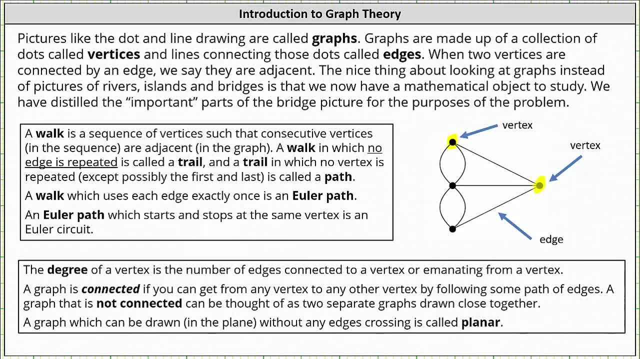 So, for example, this vertex and this vertex are adjacent, as well as this vertex and this vertex, and so on. The nice thing about looking at graphs instead of pictures of rivers, islands and bridges is that we now have a mathematical object to study. 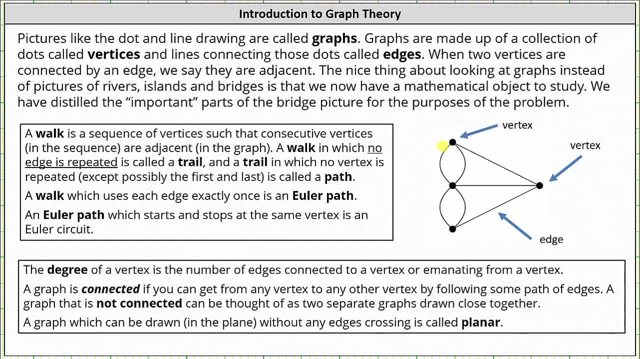 We have distilled the important parts of the bridge picture for the purposes of the problem. A walk is a sequence of vertices such that consecutive vertices are adjacent. A walk in which no edge is repeated is called a trail, And a trail in which no vertex is repeated is called a path. 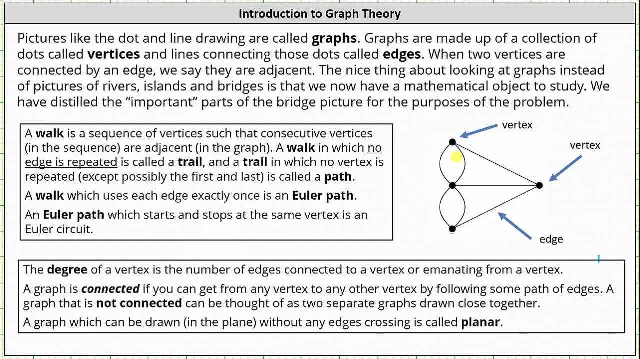 A walk which uses each edge exactly once is called an Euler path. An Euler path which starts and stops at the same vertex is an Euler circuit. The degree of a vertex is the number of edges connected to a vertex. So the number of edges is the number of vertices. 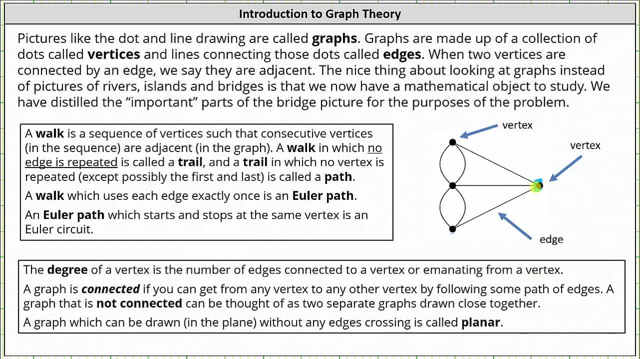 that are emanating from a vertex. So, for example, this vertex here on the right has degree three because three edges emanate from this vertex. This vertex here in the middle has degree five because there are five edges emanating from the vertex. 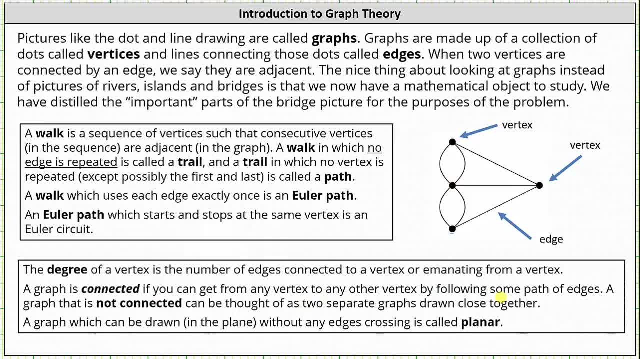 A graph is connected if you can get from any vertex to any other vertex by following some path of edges. A graph that is not connected can be thought of as two separate graphs drawn close together And finally, a graph which can be drawn in the plane. 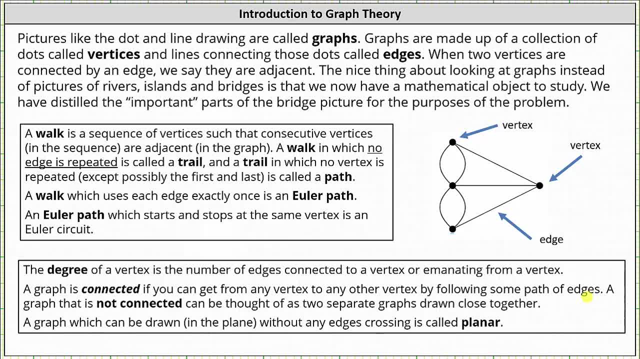 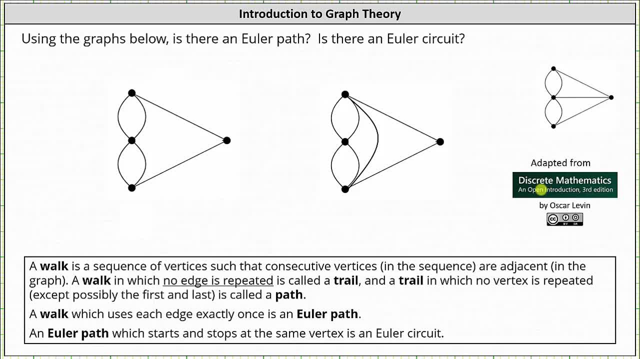 without any edges crossing is called planar. The provided graph is planar, And now let's look at an example. Use the following graphs below: Is there an Euler path? Is there an Euler circuit? A walk which uses each edge exactly once is an Euler path. 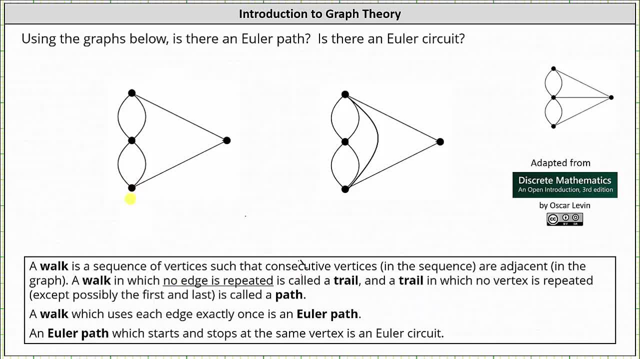 So, starting here at the bottom, let's see if we have an Euler path. So we're going to start here And we end it here. We were able to form a walk which uses each edge exactly once, and therefore the graph does have an Euler path. 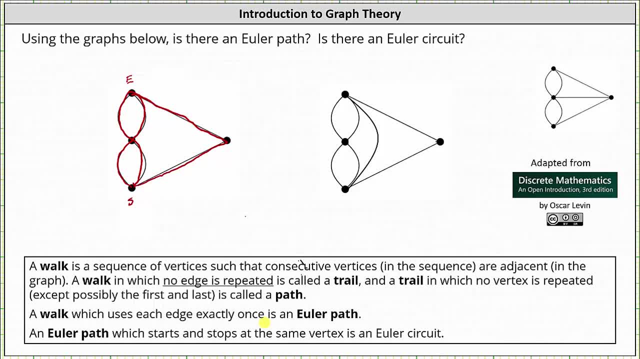 However, we did not start and stop at the same vertex. We do not have an Euler circuit. And now let's look at the second graph And again, we're going to start down here. again, Let's follow a similar walk. Notice: this time we started and ended at the same vertex. 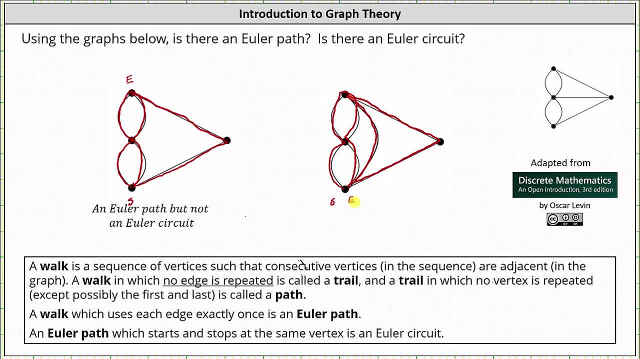 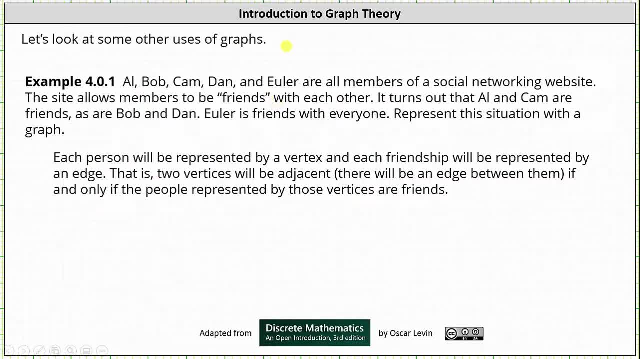 And we did use each edge exactly once. This graph has an Euler path as well as an Euler circuit. And now let's look at some other uses of graphs. Al, Bob, Cam, Dan and Euler are all members of a social networking website. 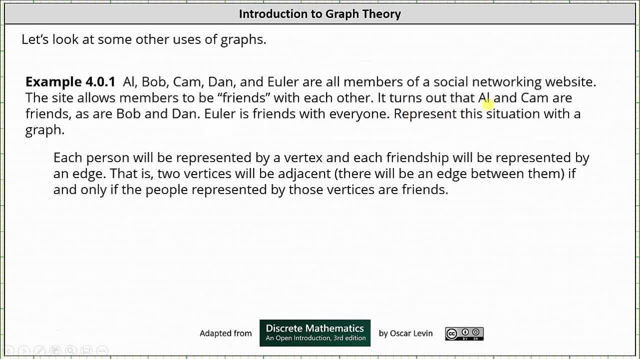 The site allows members to be friends with each other. It turns out that Al and Cam are friends, as are Bob, and Dan Euler is friends with everyone. Represent the situation with a graph. Each person will be represented by a vertex and each friendship will be represented by an edge. 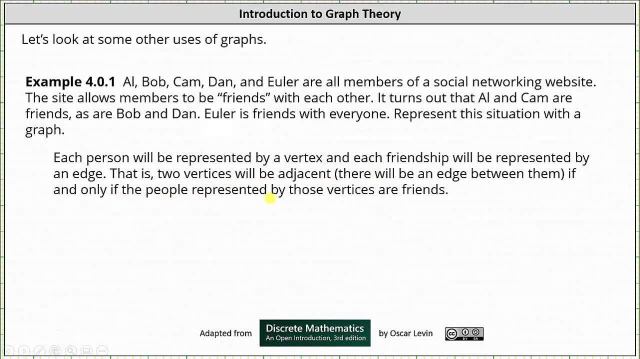 That is, two vertices will be adjacent if, and only if, the people represented by those vertices are friends. To get started, let's just list five vertices in a row and label them: A, B, C, D and E for Al, Bob, Cam, Dan Dan. 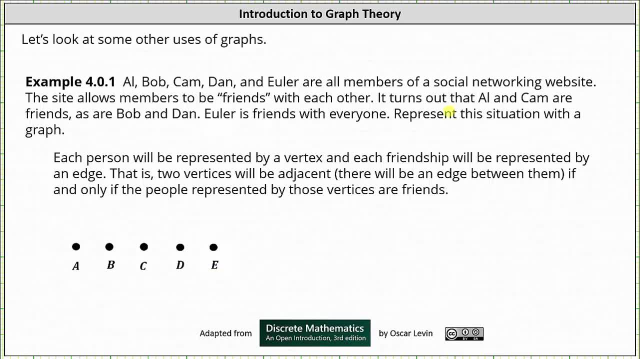 Dan and Euler From here. since Al and Cam are friends, we need an edge from A to C. Bob and Dan are friends. we need an edge from B to D. Euler is friends with everyone. we need an edge from E to D, E to C, E to B and E to A. This graph does.